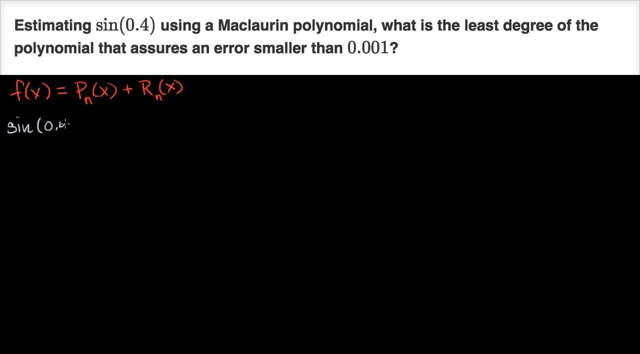 We want to say: look, if we're taking the sine of 0.4,, this is going to be equal to our Maclaurin, our nth degree Maclaurin polynomial, evaluated at 0.4, plus whatever the remainder. 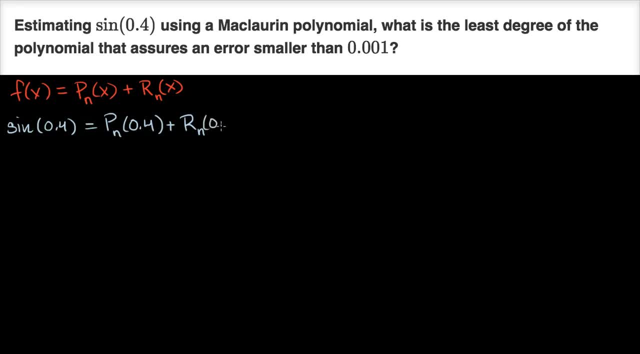 is for that nth degree Maclaurin polynomial evaluated at 0.4.. And what we really want to do is figure out for what n, what is the least degree of the polynomial. So what is? let me do this in a different color. 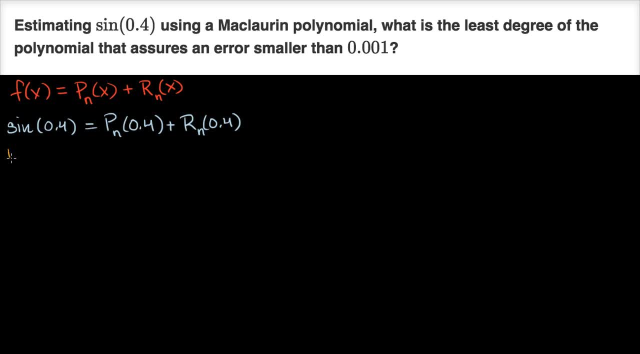 So we want to figure out what is the smallest n. what is the smallest n such that the remainder of our nth degree Maclaurin polynomial, evaluated at 0.4, is less than this number, is less than 0.001.. So this is just another way of rephrasing the problem. 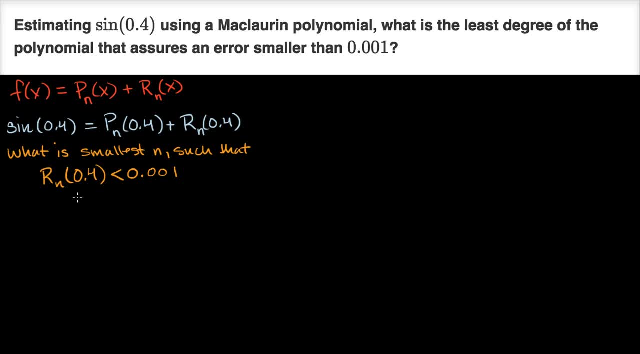 And the way that we can do it is we can use something called the Lagrange error bound, and we have other videos that prove it. This is often also called Taylor's remainder theorem, And I'll first write it out and I'll try to explain it while I write it out. 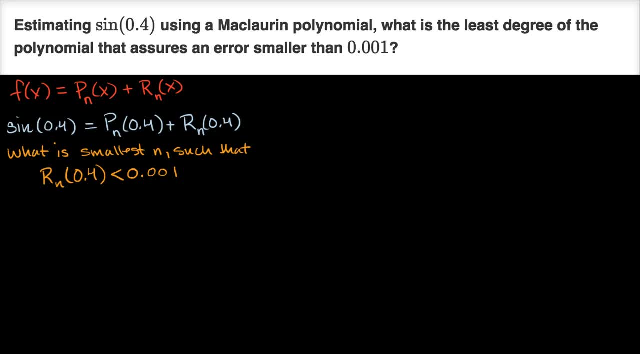 but it'll actually become a lot more concrete when we work it out. So Taylor's remainder theorem tells us, or Lagrange error bound tells us, that if the n plus 1th derivative of our function, so f, so this is our n plus 1th derivative of our function. 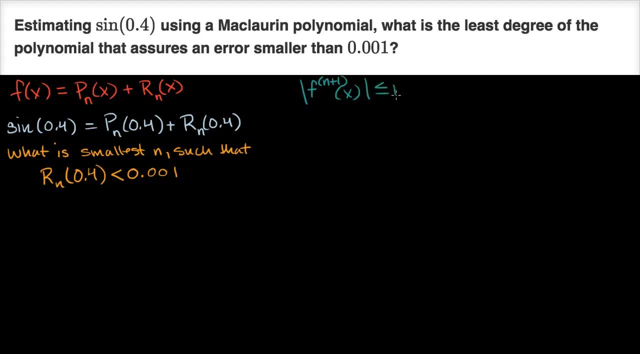 if the absolute value of that is less than or equal to some m for an open interval, which is an open interval containing where our containing, where our polynomial is centered. in this case, it's zero. We're gonna use the Maclaurin case. 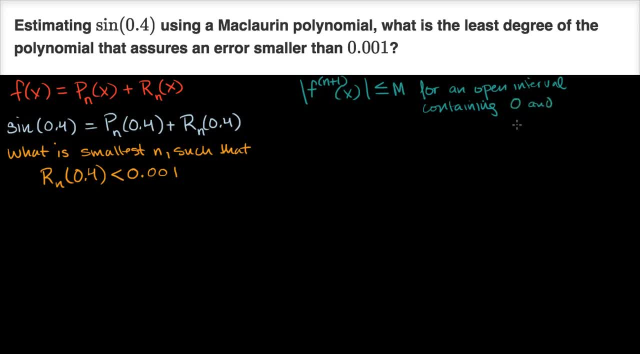 So it's containing zero and the x. that, or zero and x. the x that we care about in this particular video is 0.4,, but I'll say it in general for any x. So if this is true, if our n plus 1th derivative, 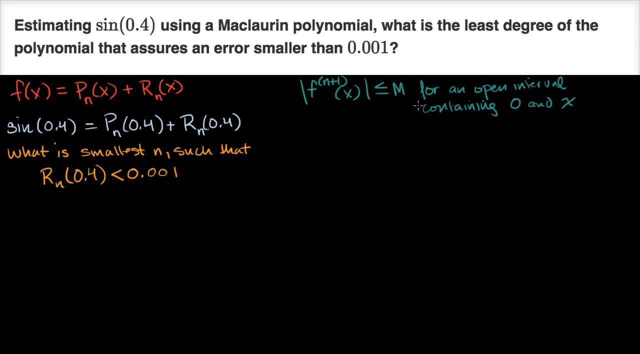 of our function if the absolute value of it is less than, less than or equal to m over an open interval containing where we're centered. this would be c if we're talking about the general case, and x. so this x right over here. 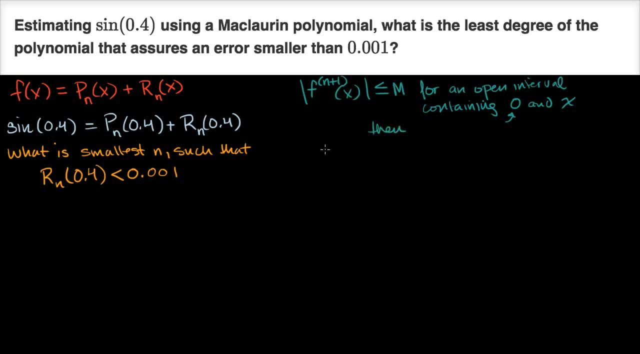 then- and this is the Lagrange, this is the part that's useful- we can say that the remainder is bounded, the remainder for that nth degree polynomial. So this is the n plus one-th derivative that's bounded. then we can say the remainder. 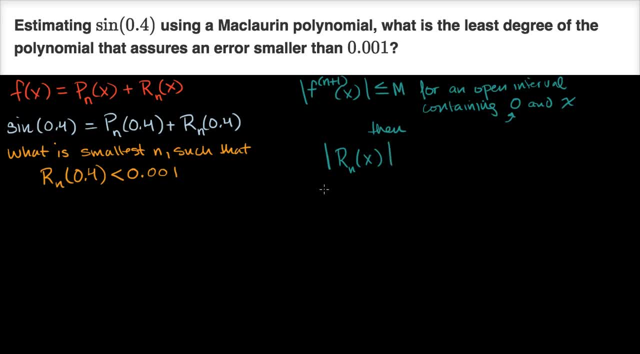 for the nth degree polynomial that approximates our function is going to be less than or equal to that: m times x to the n plus one or times x to the n plus one over n plus one factorial. So how do we apply that to this particular problem? 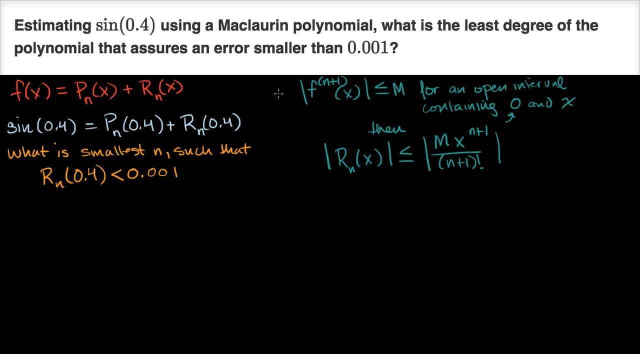 Well, think about the derivatives of sine. We know that the absolute value of sine is less than or equal to one. its derivative is cosine of x. the absolute value of that is going to be bounded is going to be less than or equal to one. 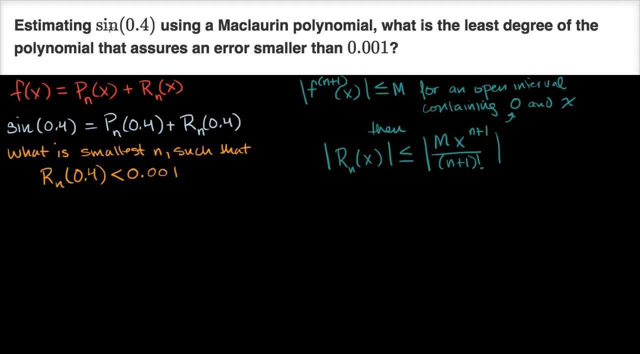 So no matter how many times we take the derivative of sine of x, the absolute value of that derivative is going to be less than or equal to one. So we could write generally that for this particular f of x. so let's say for this particular f of x right over here. 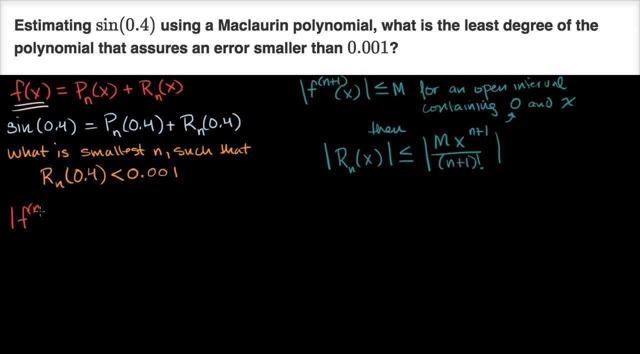 we could say that the absolute value of f, the absolute value of the n plus one-th derivative, evaluated at any x, is going to be less than or equal or equal to one. And this is the case for where f is sine, where f is sine of x. 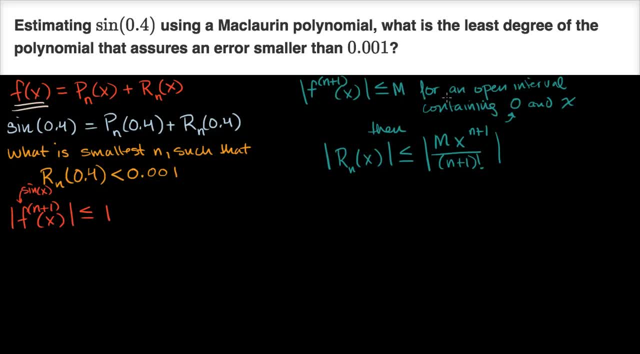 And this is actually going to be true over any interval. It doesn't even have to be over some type of a restricted interval where we can do this. So we know that this is our m, We know that this is our m, that sine and its derivatives are all bounded by 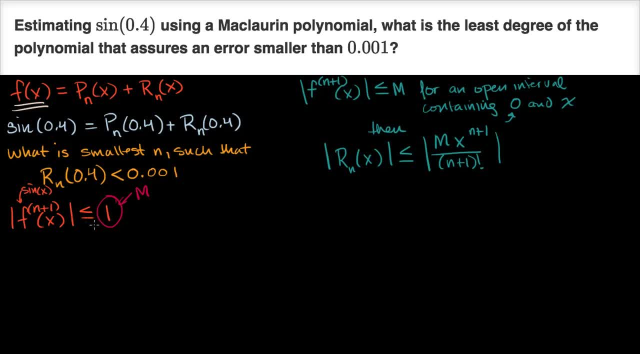 or their absolute values are bounded by one, And so then we have our m and we can apply the Lagrange error bound. So we can say that the remainder of our nth degree Maclaurin approximation at 0.4, so our x in this particular case is 0.4,. 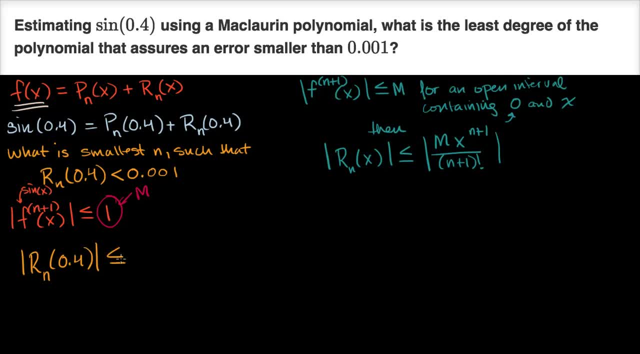 we don't have to do it generally, for any x here is going to be less than or equal to, our m is one, so I won't even write that down. our x is 0.4, 0.4 to the n plus one. 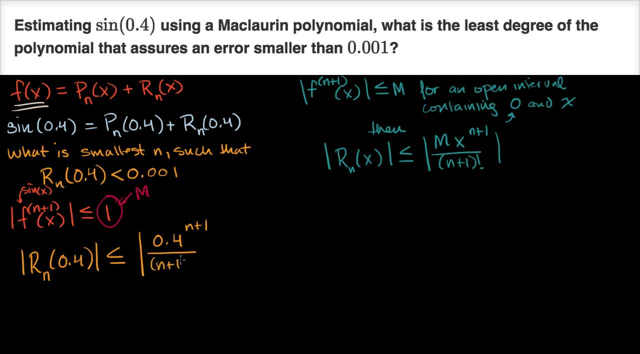 to the n plus one over n plus one factorial And we're taking the absolute value of this whole thing. This is the Lagrange error bound And we want to figure out if we can figure out a situation where this is less than 0.001,. 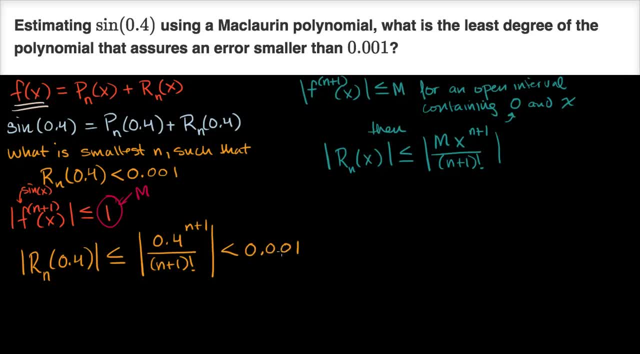 then this for sure, is going to be less than 0.001, because the remainder is less than this, or less than or equal to this, which is less than that. So how do we do that? How do we figure out the smallest n? 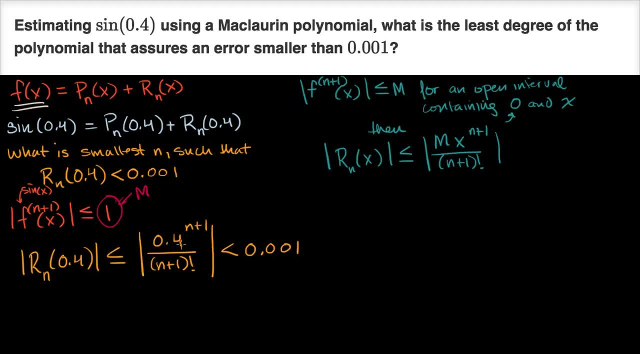 where this is going to be true. Well, we can just try out some n's and keep increasing them. Well, we can just try out some n's and keep increasing them. Well, we can just try out some n's and keep increasing them. 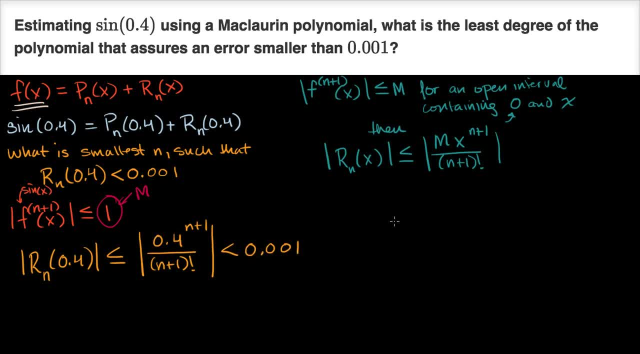 Until this thing actually becomes smaller than that thing. So let's do it. All right, I'm gonna set up a table here, So let me make a. do it relatively cleanly. So let's do. this is going to be our n. 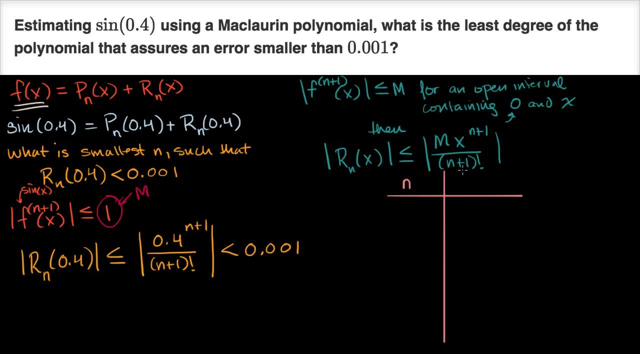 and then this is going to be: this is going to be 0.4 to the n plus one over n plus one factorial. So let's try it when n is equal to one, Well then this is going to be 0.4 to the two. 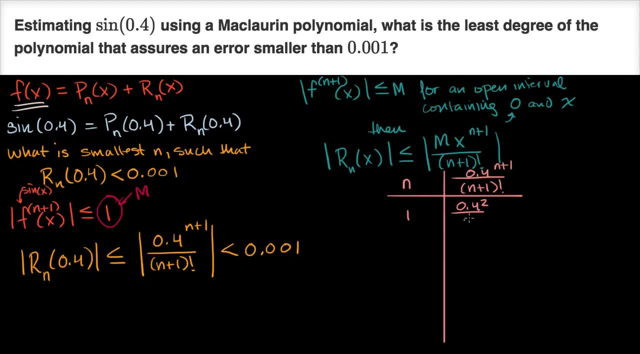 So it's 0.4 squared over two. factorial, This is 0.16 over two, which is equal to 0.08.. That's definitely not less than 1,000 here. So let's try: n equals two. When n equals two, it's gonna be 0.4 to the third power. 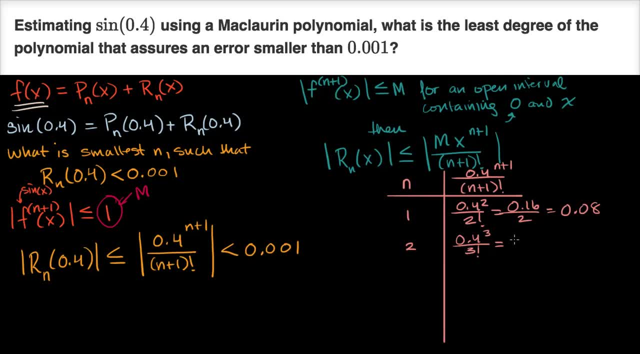 over three factorial, and that's equal to what? is that Zero point? I'm gonna need three digits behind the decimal: 0.064 over six. Well, this is a little bit more than 0.01.. So this isn't our n isn't large enough yet. 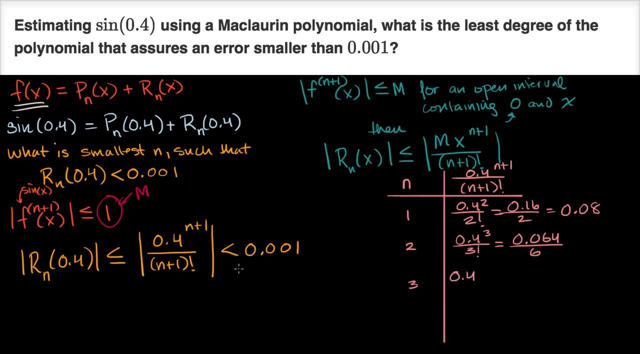 So let's try three. So this is going to be 0.04 to the three plus one, So that's going to be to the fourth power over four factorial and let's see that is going to be equal to. this is going to be: 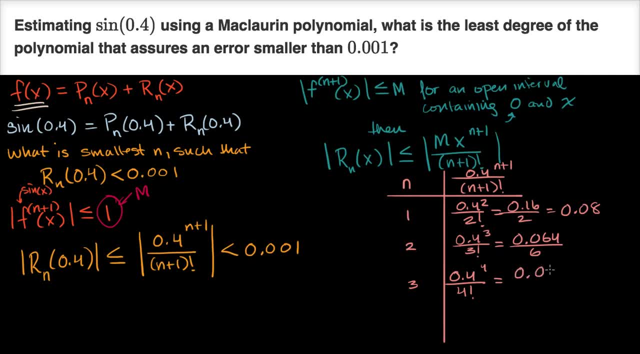 let's see. So this is going to be four digits behind the decimal, So 0.0256 over 24.. This is we're almost there. This is a little bit. this is going to be a little bit more than 0.001..